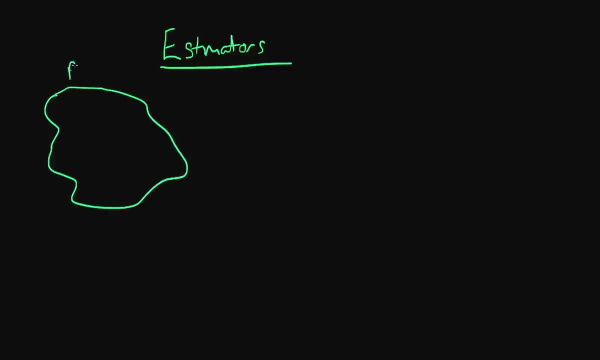 So, in general, we have a population. So we spoke about what this could be before. so this could be a population of all the countries in the European Union. for example, It could be a population of products which a company sells, And the example which I'm going to talk about here is going to: 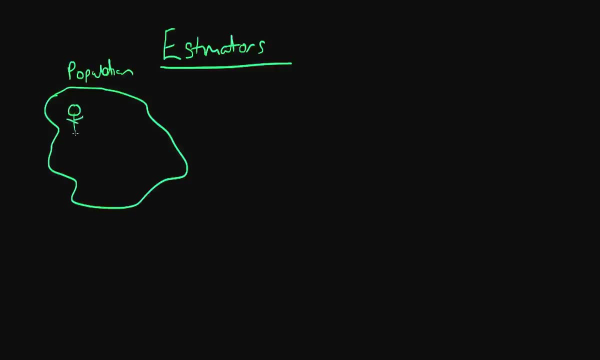 be the under 18 population within the UK And we spoke about how there might be some underlying population process whereby, on average, there is an effect which one year of education- well, an incremental effect of one year education has on wages, Which is given here in a population by beta, or I'm actually calling it beta p. 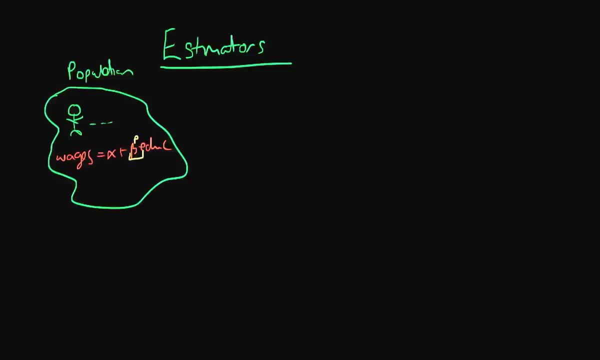 In general. however, we don't have an entire population of data, We only have a sample from that. So let's say we might have sort of a thousand individuals. I'm not saying we get all our individuals just from this one particular spot. Maybe we get one from here up in the north of. 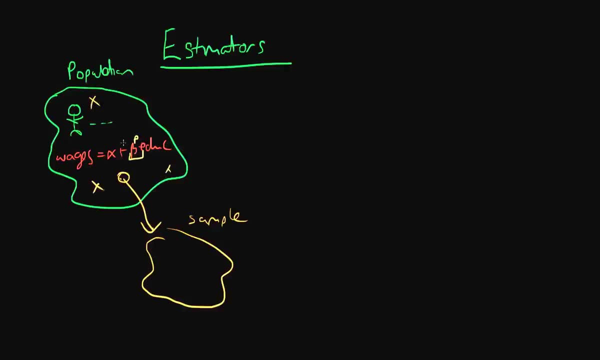 England, Maybe we get one from here in Wales, etc. And I'm just saying that we don't have the full amount of population data to work with And in this sample we need to figure out a method which uses the sample data to estimate what this or to come up with an estimate of the population. 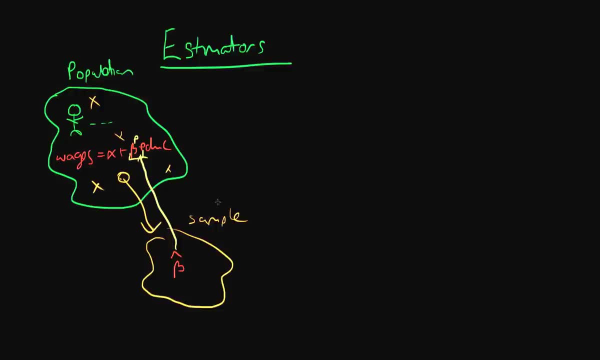 parameter, And what we do is in econometrics is something which we call estimators. So what is an estimator? Well, the idea with an estimator is that you feed in sort of sample data to this thing which I'm going to call beta hat. Normally, we use hats when we're talking about estimators, And so this is. 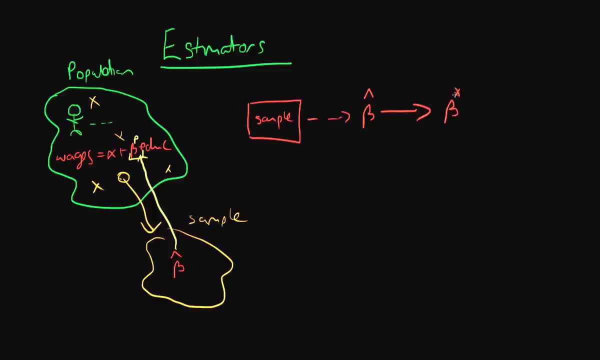 the sample data is fed in as an input and then it outputs an estimate of our population parameter. Note that there is a difference between an estimator, which is in general some sort of mathematical function, and beta star, which is just a sort of point estimate of the population.